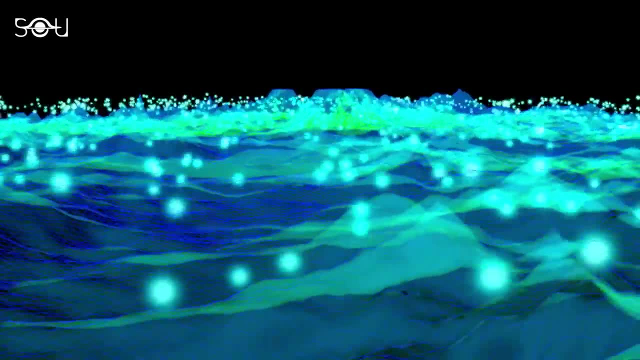 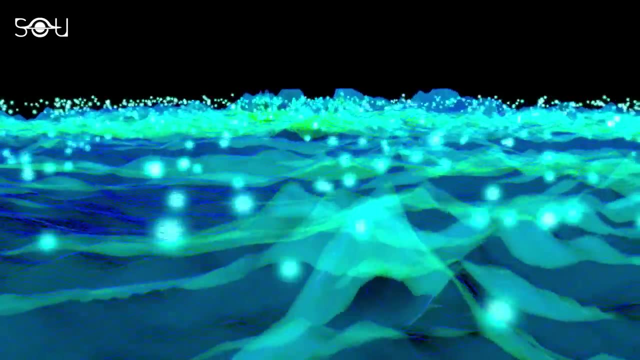 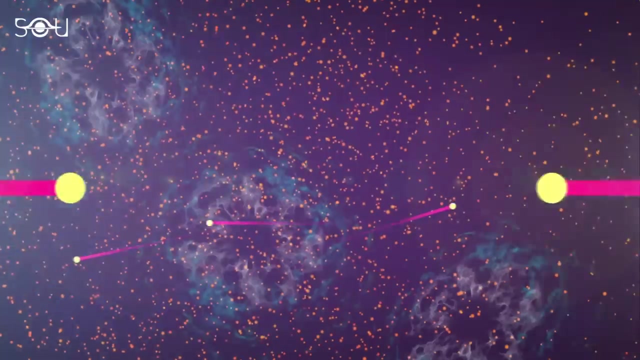 According to the quantum field theory, the vacuum isn't really empty. Instead, it is full of virtual particles which emerge and vanish in pairs out of nowhere in space. These virtual particles cause vacuum fluctuations, In other words, they cause a random change in the amount of energy in space. 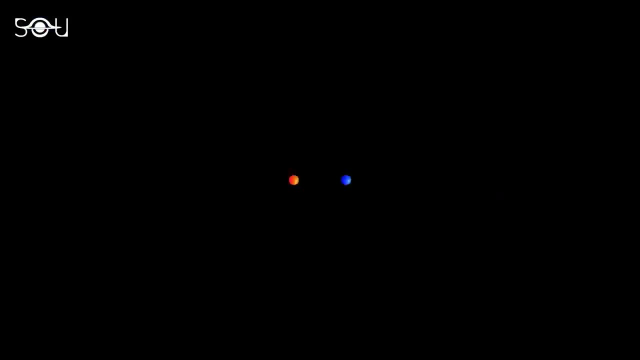 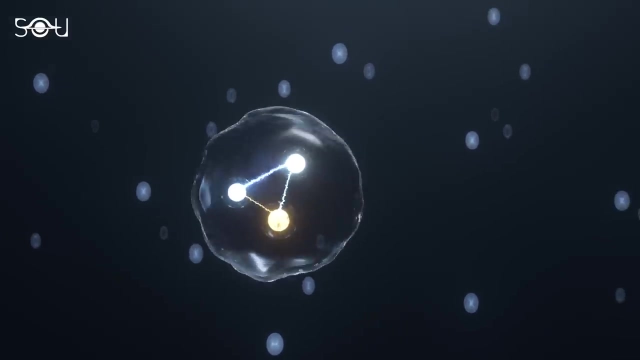 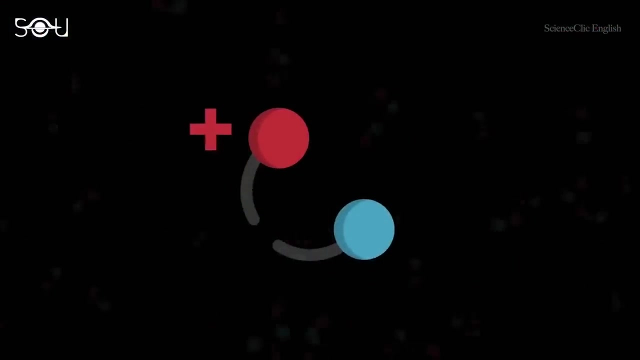 The virtual particles always appear and vanish in pairs of a particle and an antiparticle. Since these particles appear without a source of energy, they are said to violate the energy conservation law. When a pair of particles is isolated, one of the particles has positive energy whereas the other one has negative energy. 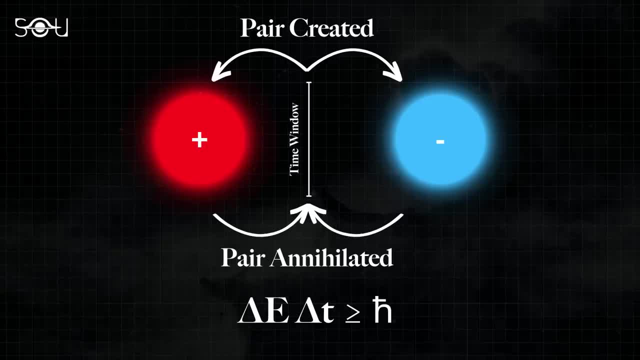 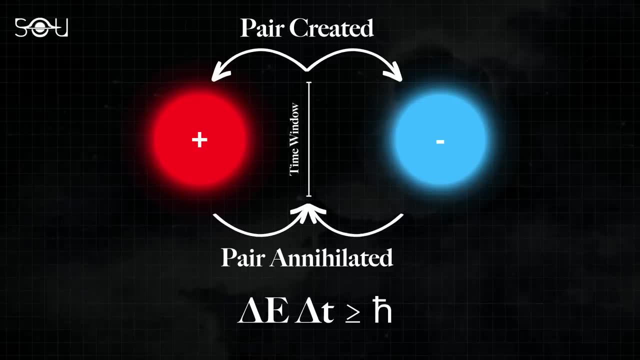 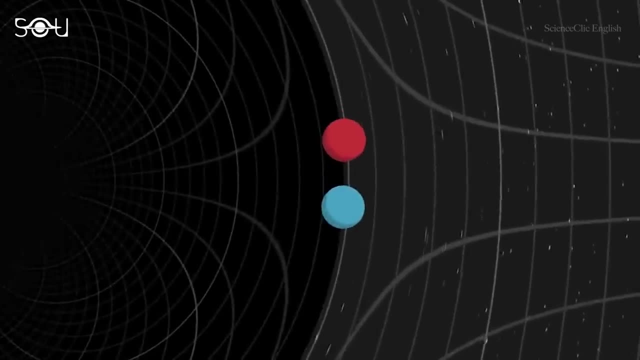 Although the net energy of the pair is still zero. this can cause a violation of energy conservation, But this is theoretically allowed because the particle and antiparticle annihilate each other within a time window provided by the energy time Heisenberg principle. However, there is another twist. Sometimes the negative energy particle crosses the event. 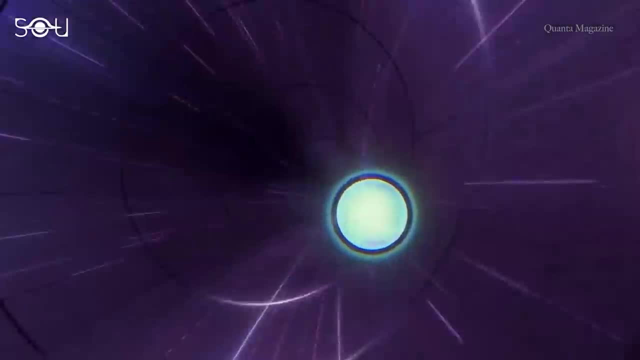 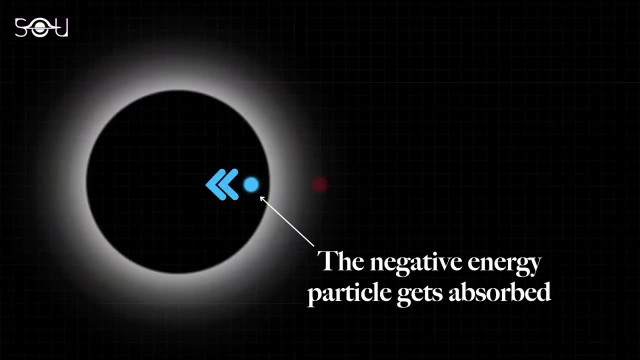 horizon gets absorbed by the black hole, but on one condition: that the particle moves radially inwards towards the black hole. so the negative energy particle from the vacuum fluctuation gets absorbed by the black hole without violating the uncertainty principle. In contrast, the positive energy particle is freed and escapes into infinity. 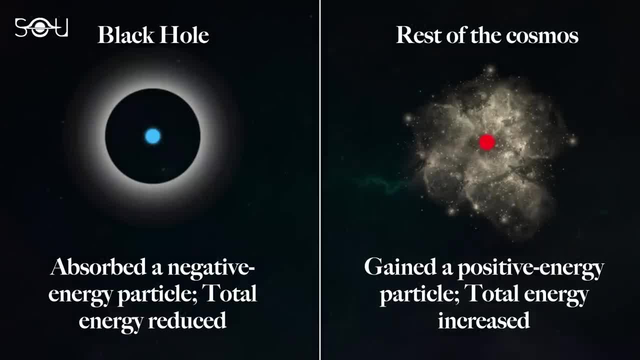 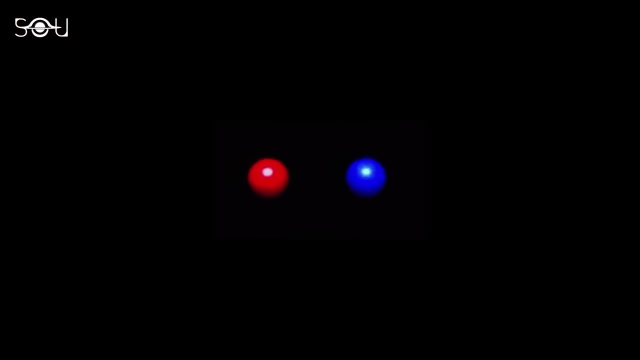 As a result, the black hole loses energy to the vacuum fluctuation due to the negative energy particle, whereas the energy of the rest of the universe increases because of the positive energy particle. But this still does not sit right, because how is it possible that a pair of particles 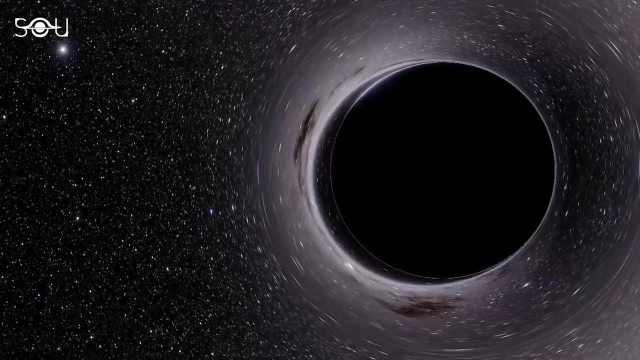 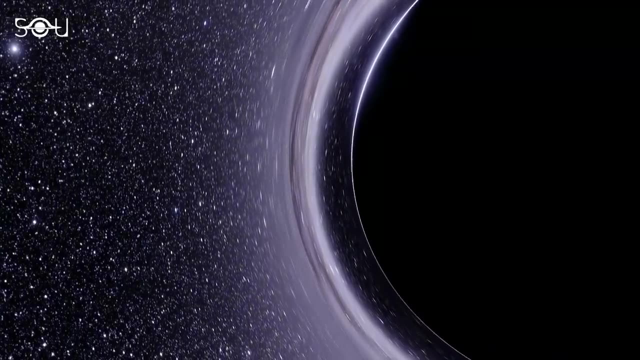 is created out of nowhere. The answer to this is the black hole's intense gravity. These particles are believed to appear near the event horizon of the black hole due to disturbance in the spacetime caused by the black hole's strong gravity. But, more importantly, 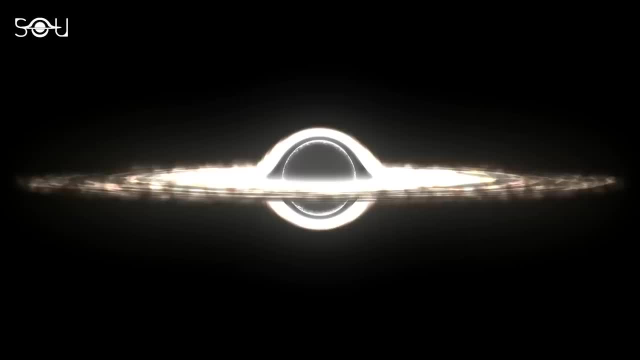 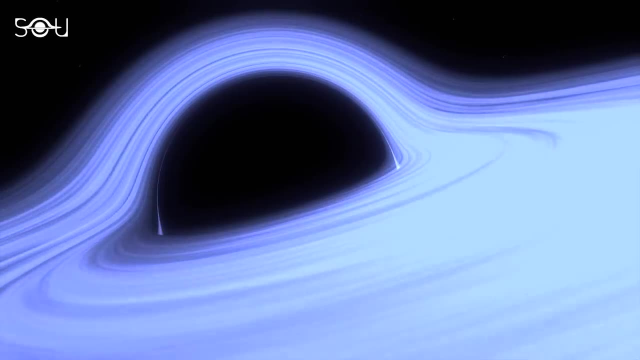 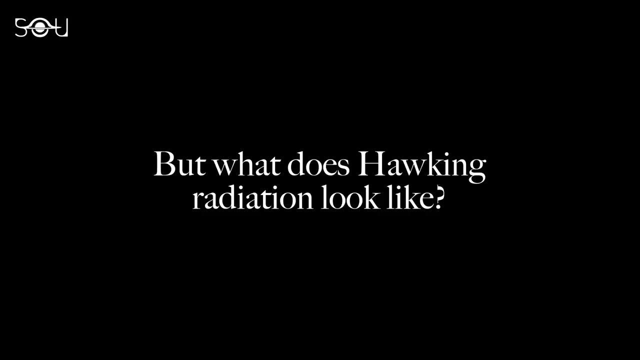 the mass of the black hole itself is converted into energy that escapes out of the event horizon. Therefore, Hawking radiation reduces the mass and energy of the black hole. To understand what the researchers did, it's important to know the nature of Hawking radiation. 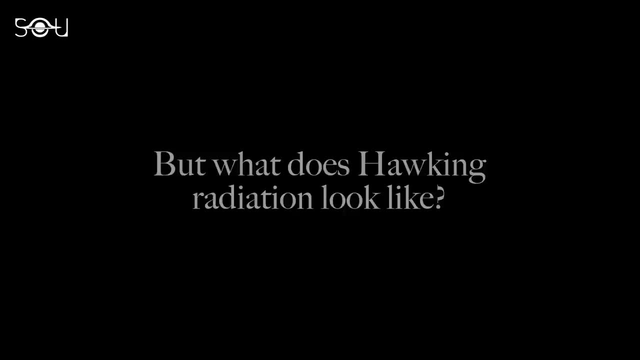 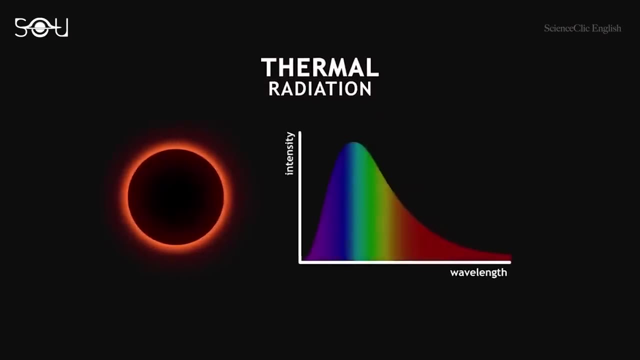 in the first place. So what does it look like? Hawking radiation acts like a black body, radiation with a Planck spectrum, meaning the nature of thermal radiation being emitted by the black hole. So what does it look like? In theory, the mass of the black hole is similar to that of radiation from a star. 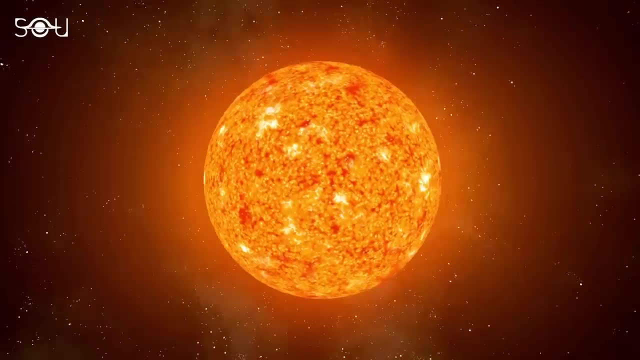 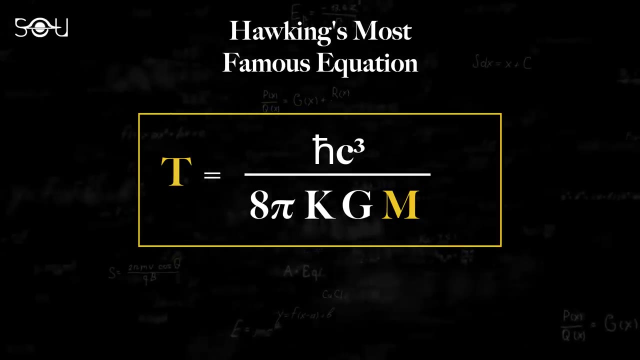 The phenomenon of a black body radiation is similar to that of radiation coming from a star, But in fact this is important because it means that the temperature of the radiation is inversely related to the mass of the black body. So the larger a black hole, the lesser its temperature and the longer it will take to. 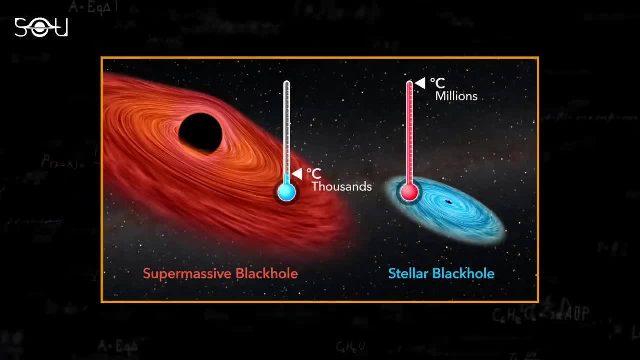 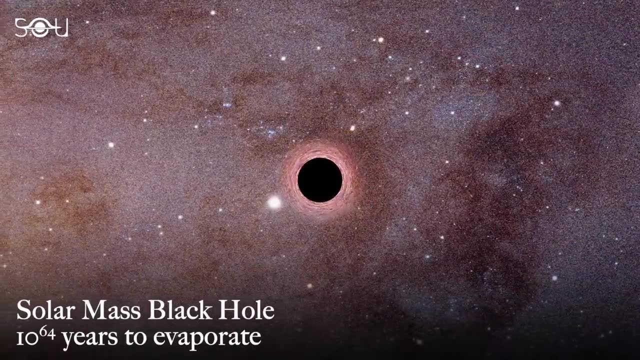 evaporate. For reference, a solar-mass black hole would take ten rays to the power- sixty-four years to evaporate. On the other hand, a supermassive black hole with a mass of one hundred and twenty degrees would take an additional thousand years. 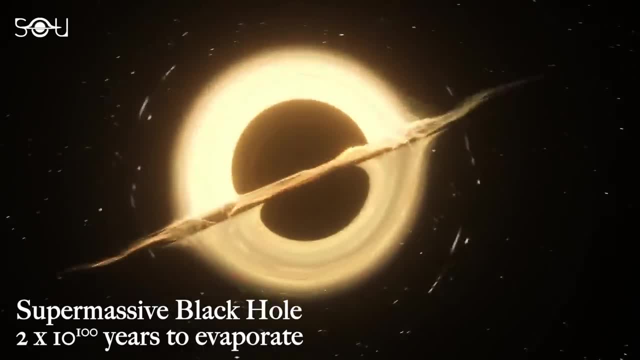 The prepare for the black body reaction is usually connected to the mass of the black body and draußen and Rebel energy. However, a solar mass black hole would take a total of forty years to get out of the black hole, 100 billion solar masses would evaporate in 2 into 10 rays to the power 100 years. 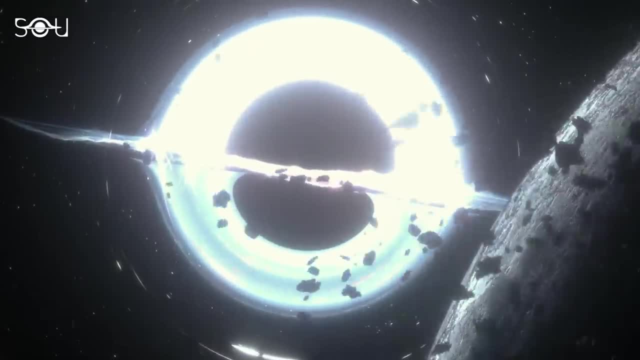 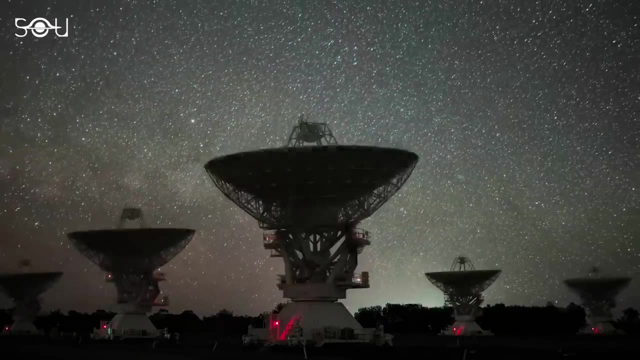 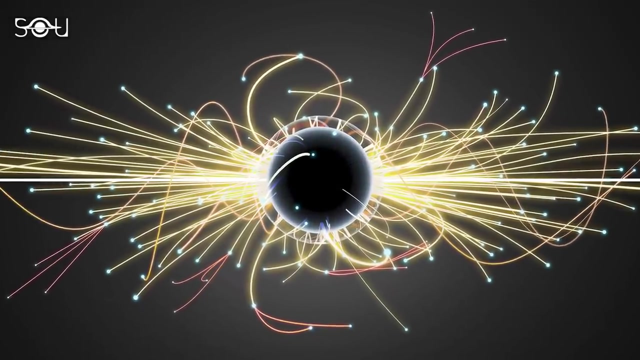 Hawking radiation has remained elusive for a long time because it's too faint to detect from supermassive black holes. However, since its discovery can lead to groundbreaking results in physics and astronomy, scientists tried to study its nature through lab-grown black hole analogues. 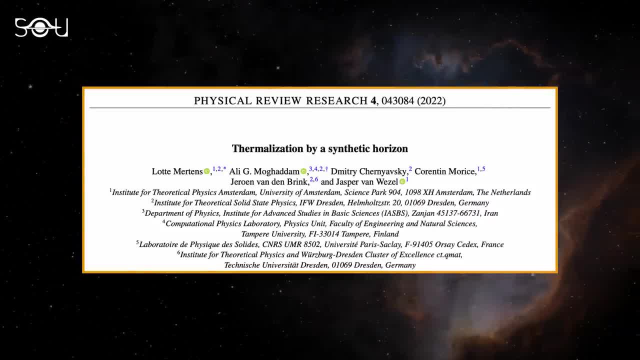 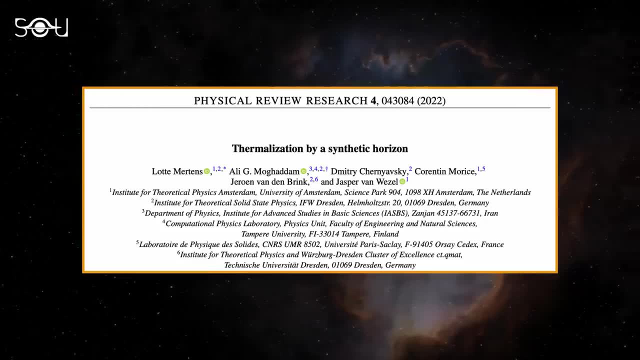 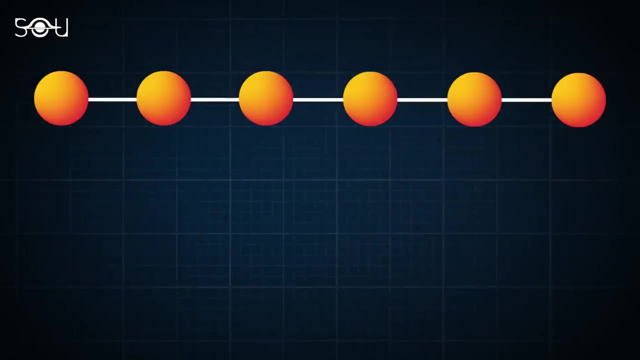 A team from the University of Amsterdam conducted a detailed analysis of Hawking radiation from the synthetic horizon by changing certain conditions to make Hawking radiation purely thermal. To begin with, they created a one-dimensional chain of atoms for electrons to hop from one atomic site to another to replicate the hopping of particles around the event horizon. 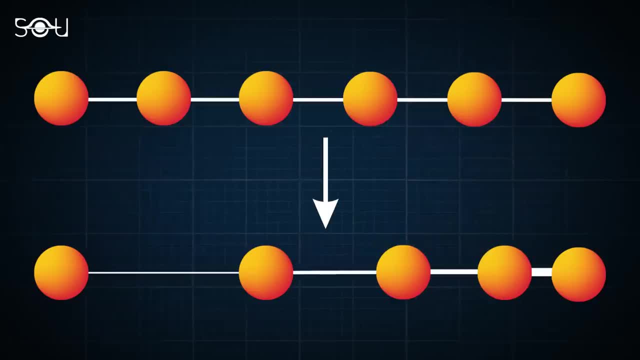 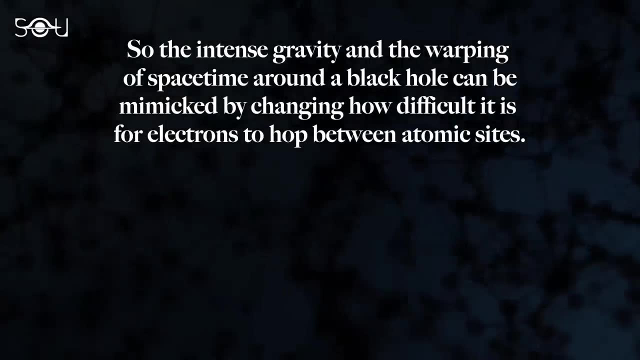 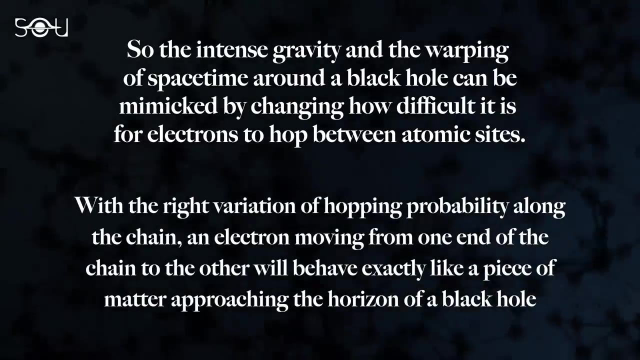 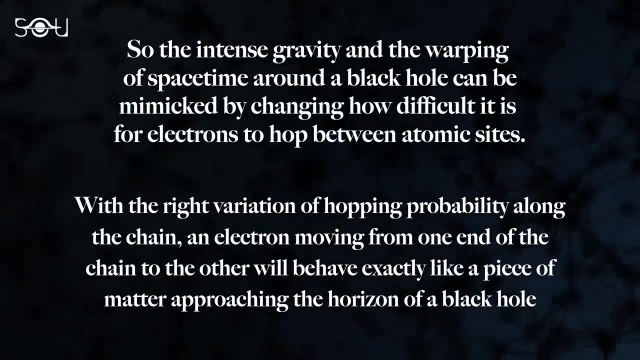 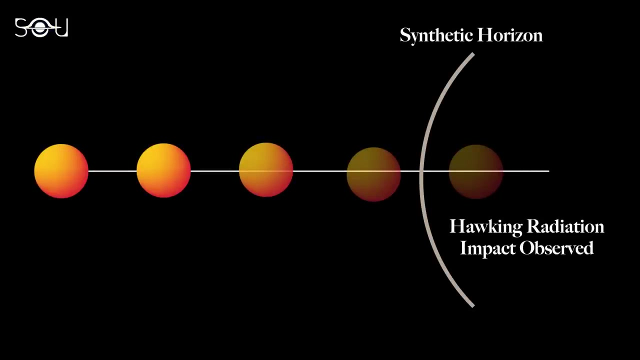 The warping of spacetime due to the presence of a black hole was mimicked by tuning how easily electrons can hop between each site. Through this, they could create a synthetic event horizon. When the team extended the chain of atoms beyond the synthetic horizon, the effect of 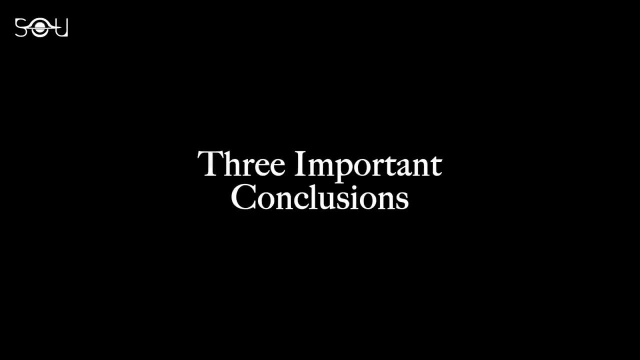 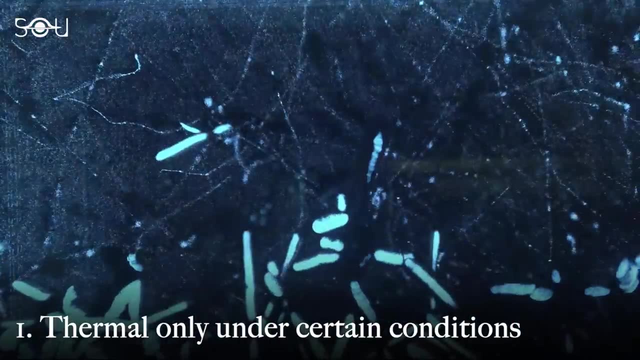 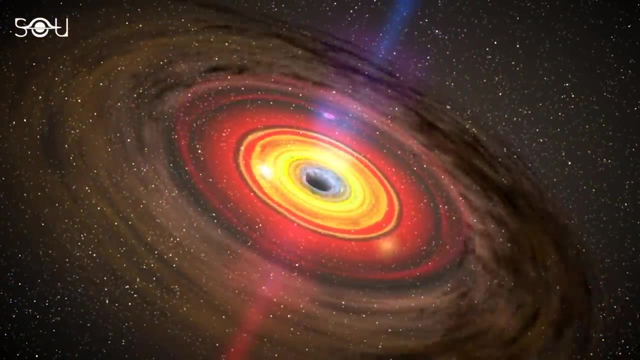 Hawking radiation was seen 4.. There were three critical conclusions from this experiment. The first is that the radiation was thermal only under specific conditions of spatial variation of the hopping probability, which means that real Hawking radiation may also only be purely thermal in certain situations. 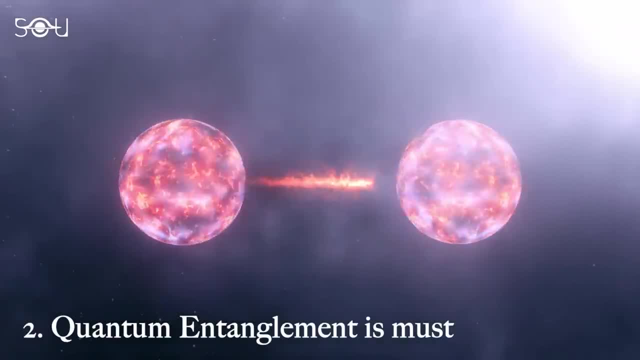 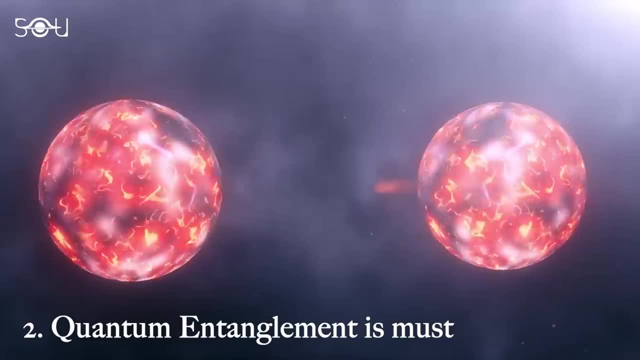 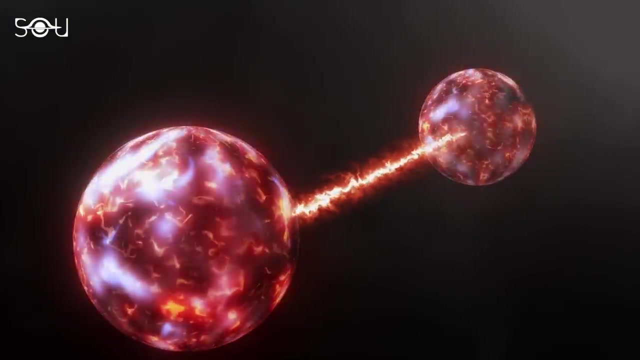 The second is that entanglement is necessary for Hawking radiation. The entanglement of particles is essentially a quantum mechanical effect that explains how two particles are linked despite their vast separation. The team observed that Hawking radiation is directly connected with an entanglement between 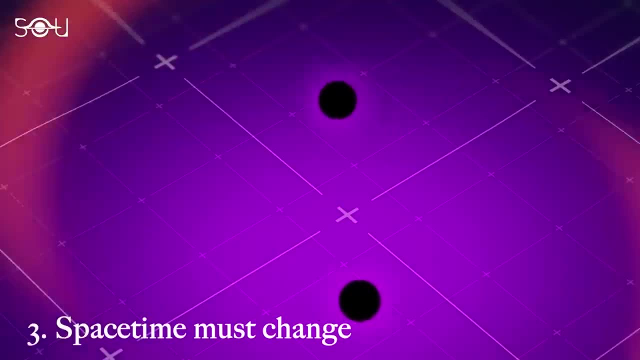 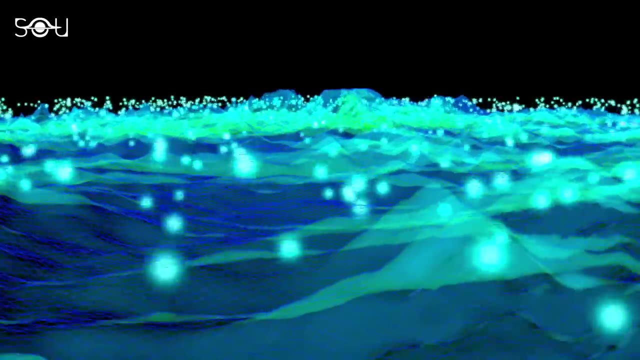 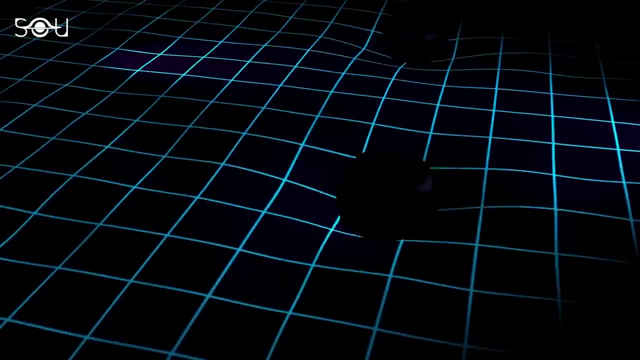 objects on either side of the horizon. Finally, they concluded that Hawking radiation requires a change in the warping of spacetime. It only occurred when the model system started without any spatial variation of hopping probabilities, mimicking flat spacetime without any horizon, before it was changed. 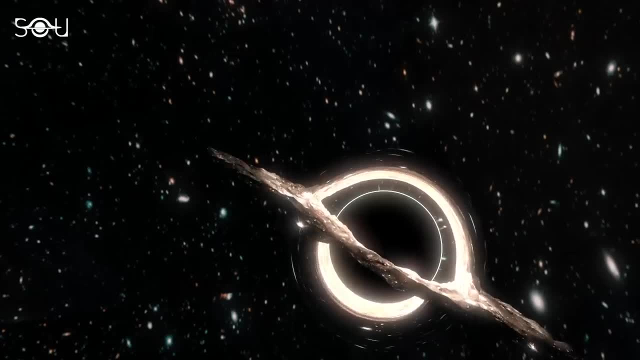 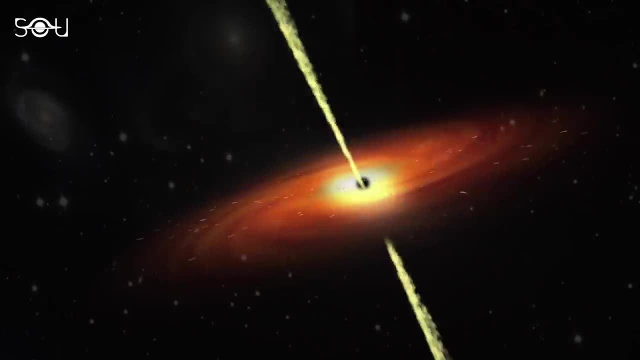 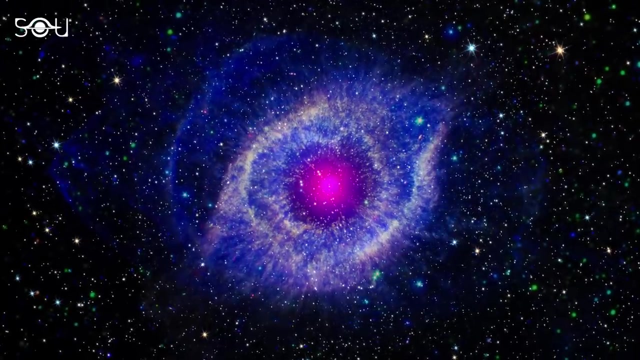 So what is Hawking radiation? As exciting as Hawking radiation sounds, some implications impact the rest of the universe First, through Hawking radiation, a black hole interacts with the universe. As its mass keeps reducing, the energy of the universe keeps increasing. 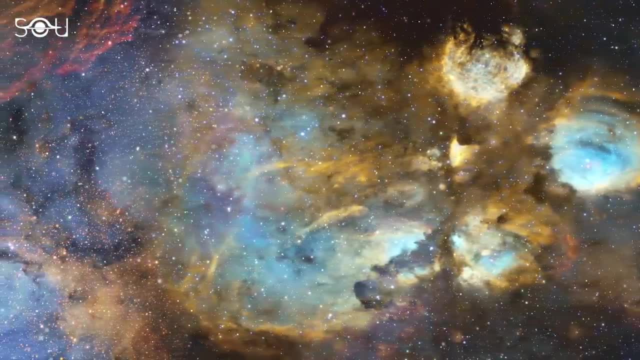 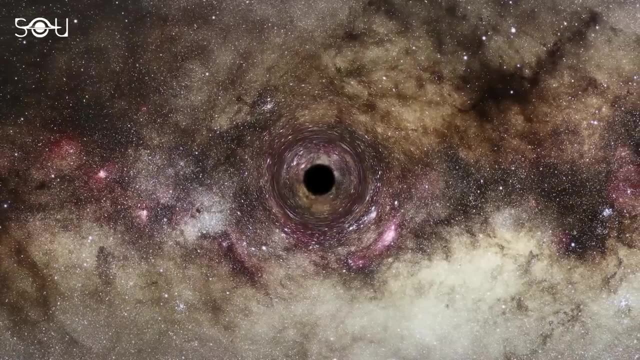 This is how black holes thermally interact with the universe. Second Hawking radiation leads to the evaporation of the black hole. If the black hole is isolated, the black hole will not move. If the black hole is isolated and not feeding on any surrounding star, it is eventually. 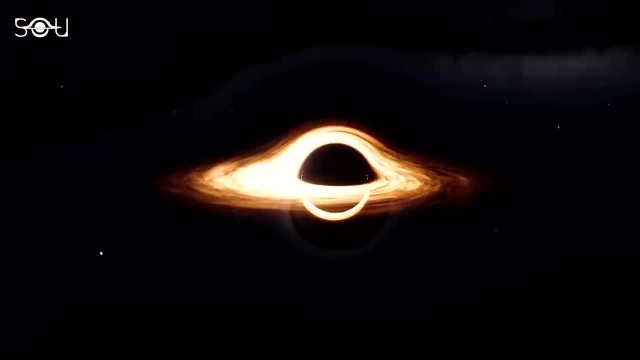 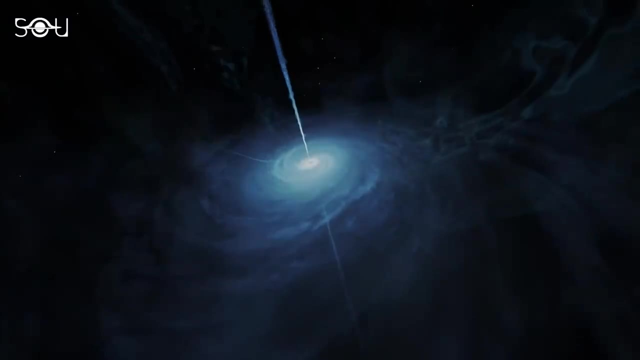 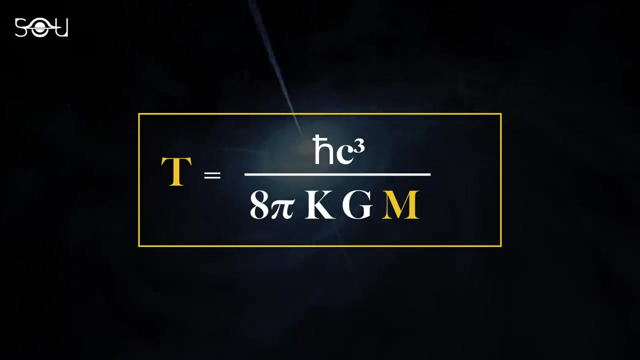 reduced to nothing. So Hawking radiation implies that black holes are not eternal objects of the universe. With time they too will vanish. But an interesting thing happens near the end of the black hole. Since the temperature of the radiation increases with decreasing mass of the black hole, the 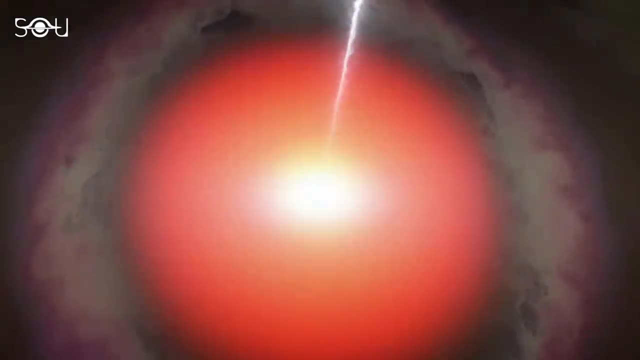 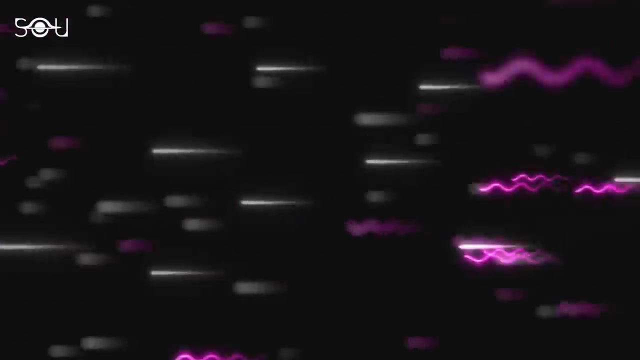 radiation temperature skyrockets towards the end. Such black holes with low mass are most likely to emit high-energy radiation In the form of powerful jets of particles, So the endpoint of black holes is most likely violent explosions in the form of X-rays and. 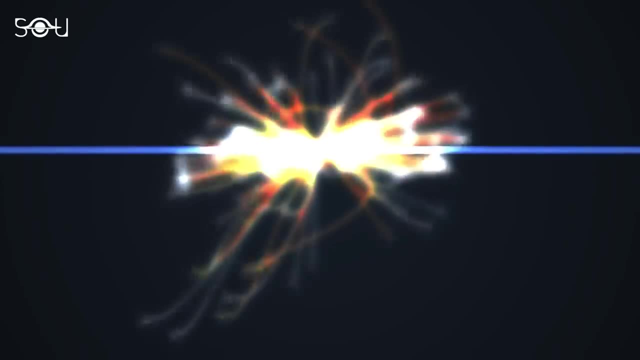 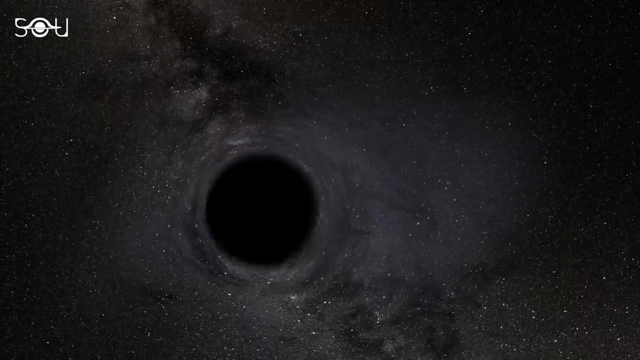 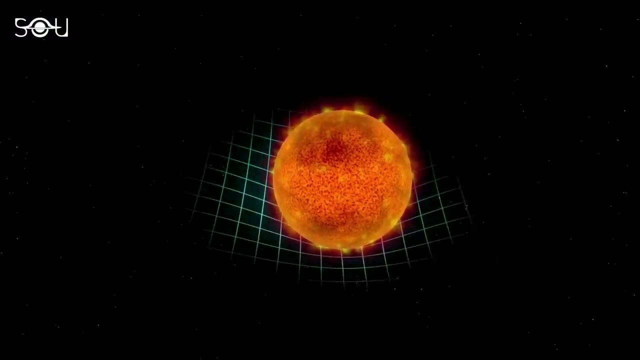 gamma rays. The study of Hawking radiation could open new windows into high-energy physics and astroparticle physics In the bigger picture. studying analog black holes and Hawking radiation will pave the way to explore the interplay of quantum mechanics and the gravitational field that may lead.